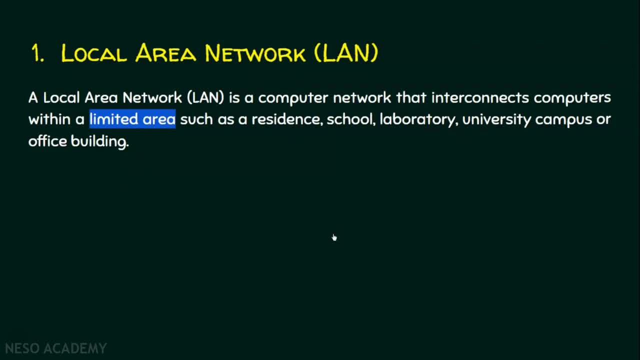 university campus or office, say a small network that is there in our residence or our school, lab, university campus or office, say a small network that is there in our residence or our school, lab, university campus or office is said to be a local area network. 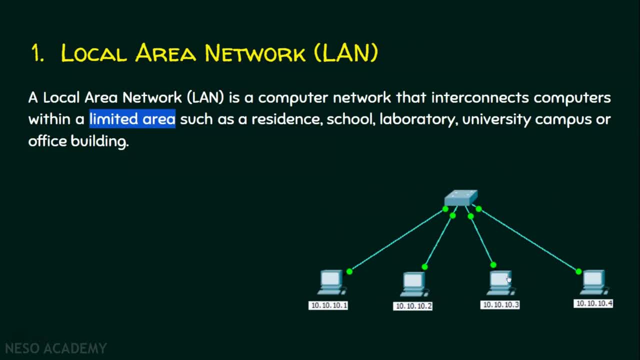 Let's take an example. Let there are 100 computers in a network, And this is a school network. Each of these computers are connected to each other with the help of a switch And we can call this computer network as a local area network. 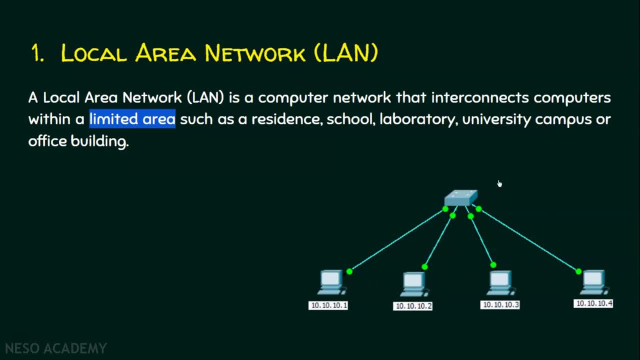 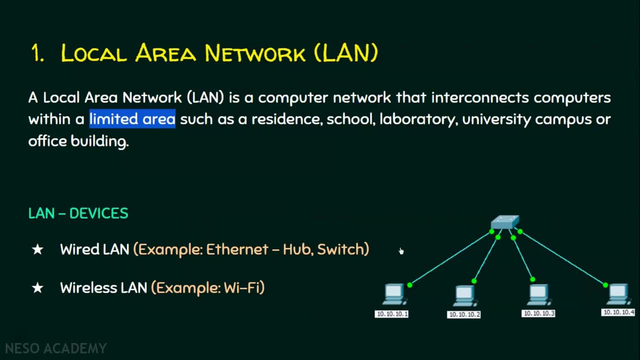 Why? Because all these computers can communicate with each other internally. We can set up LAN in two ways. One is a wired LAN, another one is a wireless LAN. In wired LAN we have cables, So the example technology is a wireless LAN. So the example technology is a wireless LAN. 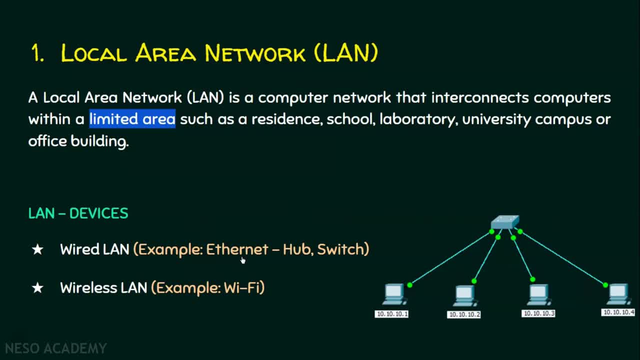 So the example technology for a wired LAN is Ethernet. We have already seen in the previous lecture that Ethernet is used to connect two or more nodes. In this case, this node is connected to the switch. This computer is connected to the switch with the help of an Ethernet cable. 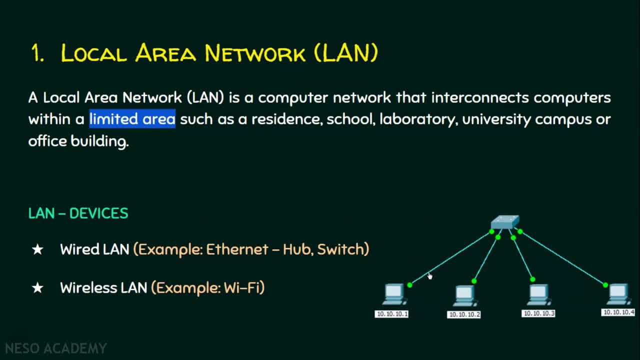 To be precise, this is an Ethernet straight-through cable, because Ethernet straight-through cable connects devices of different kinds. Switch and computers are different kinds of devices, So we need to use Ethernet straight-through cable In case if we want to connect this computer with this computer. 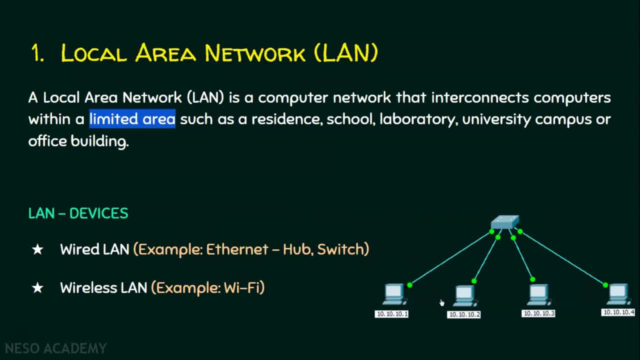 We need to connect this computer with this computer, So we need to use Ethernet straight-through cable directly. then we have to go for Ethernet crossover cable, Whatever it is. Ethernet is the well known and the most popular technology in wired LAN, And the devices that are used in the wired LAN are: 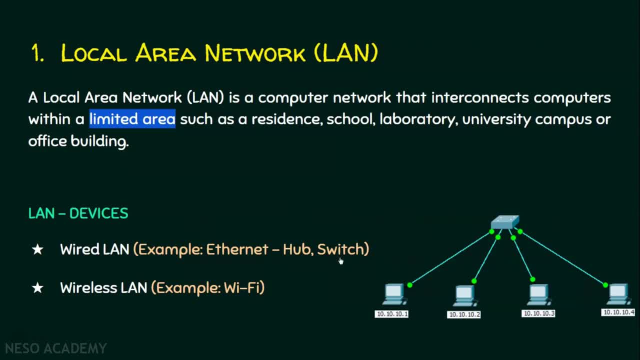 hub and switch. I will talk about this hub and switch in the next lecture elaborately. Now you just understand. hub or switch can be an intermediary device in a local area network, and that too in a wired local area network. We can also have a local area network wireless, example Wi-Fi. 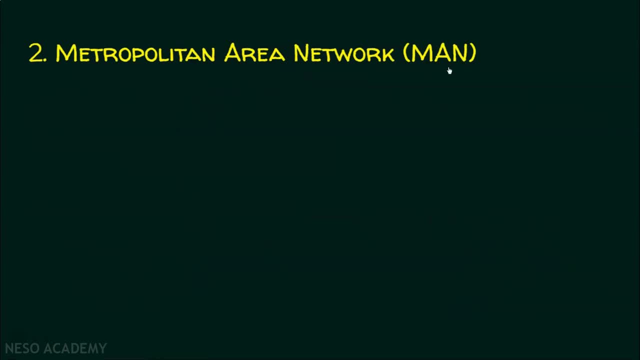 Now we will see metropolitan area network, or simply MAN. A metropolitan area network is a computer network that interconnects users or computers in a geographic region. See, there are two branches in a city and these two branches are somehow connected with each other. 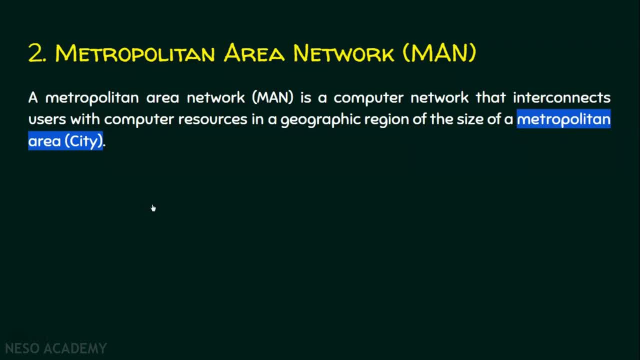 So this kind of network is called as a metropolitan area network. In other words, there are two local area networks. These two local area networks are connected to each other in a city. The devices that are used in the wired LAN are hub and switch. 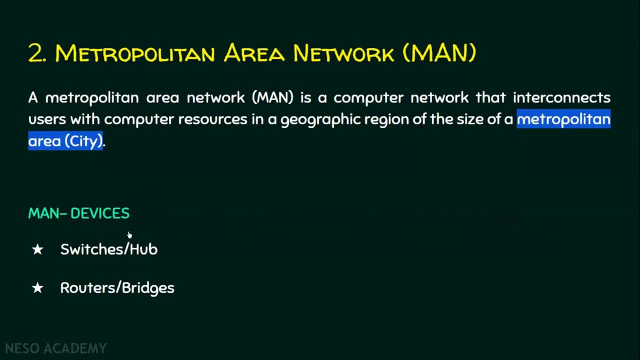 So the devices involved in this metropolitan area network are switches, hubs for establishing a local area network, And to connect two local area networks we need routers or bridges. As I already mentioned, there are minimum two local area network and these two local area networks are to be connected with each other. 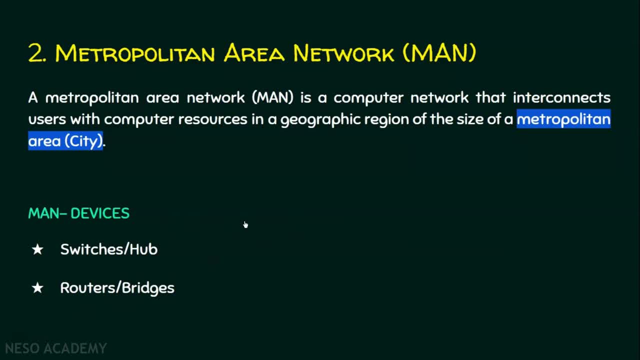 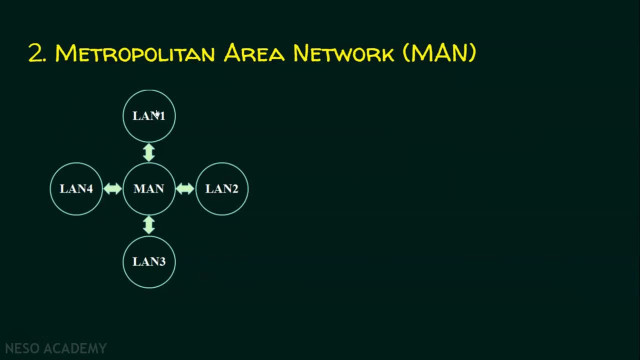 with the help of a router or a bridge. We'll see an example now. There are four local area networks connected to each other. Let's take: this is a supermarket and this supermarket has four branches. Computers in one supermarket has four branches. Computers in one supermarket has four branches. 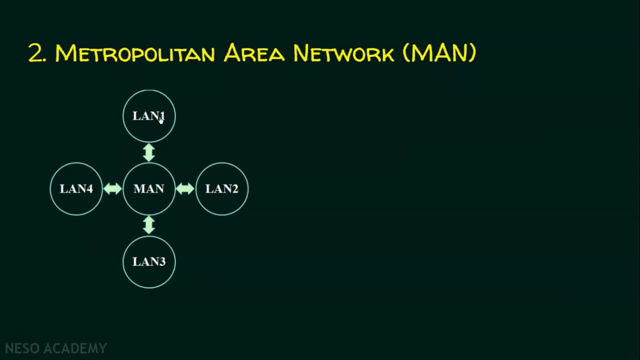 The market will be in one local area network. Similarly, other branches also have separate local area network And these supermarket branches must somehow communicate with each other. For example, if someone is asking for a product which is not there in this branch, the employee of this branch wants to search whether the product is available in other branches. 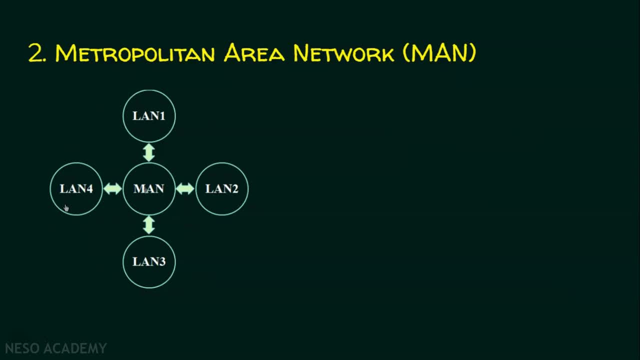 This is possible only if all local area networks of the supermarket are connected, And this is what exactly? a metropolitan area network. Please remember, this is restricted. This is restricted to only a small geographic region, like a city. Please note, in every land there are some computers. 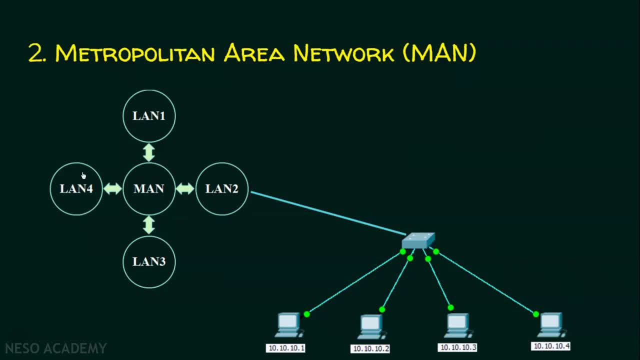 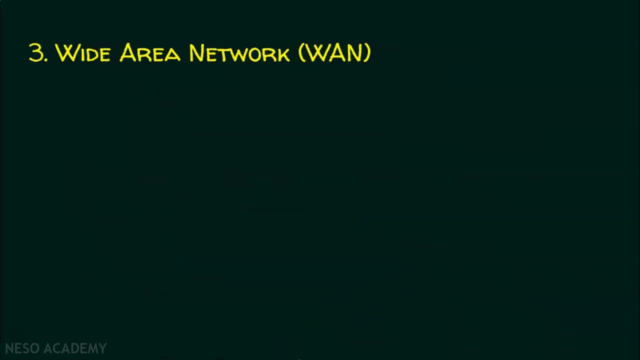 and these computers can communicate with other computers in other local area network, And this is possible only if these computers are somehow connected with each other. Time to see wide area network, that is the WAN. A wide area network is a telecommunications network that extends over a larger geographical area. 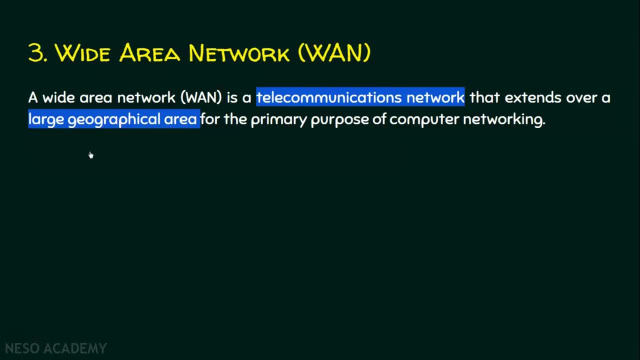 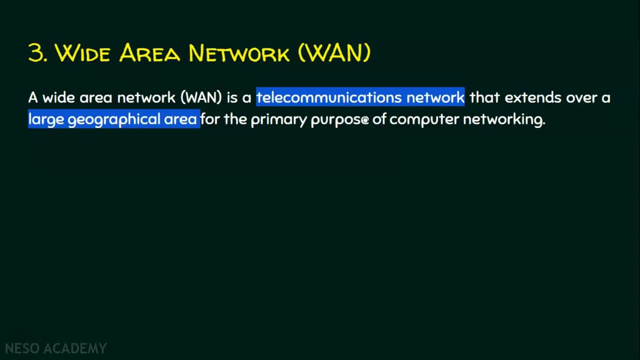 Any communication at a distance. we call it as a telecommunication network. So here the communication is going to be within a large geographical area. In WAN, two or more lands within a city can communicate with each other. In WAN, two or more lands within a country can communicate with each other. 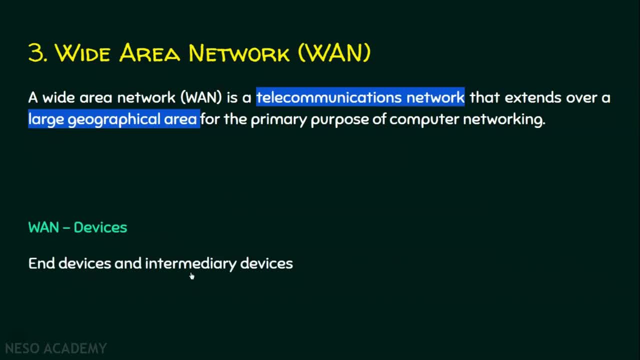 And the devices in WAN are all end devices are connected to each other. And the devices in WAN are all end devices are connected to each other Because an end device in one part of the country may want to communicate with an end device which is in the other part of the country. 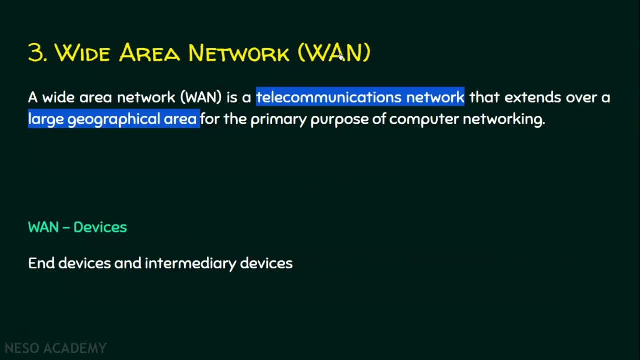 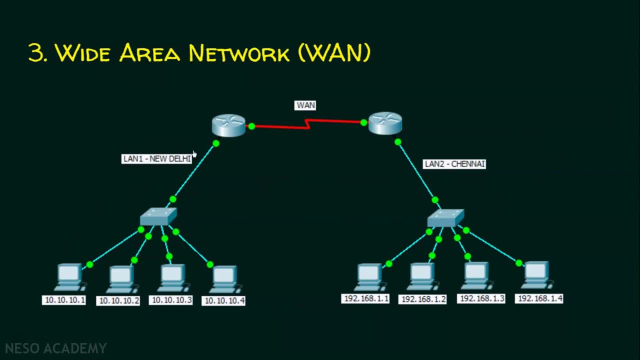 And some authors will refer this wide area network to be the internet. We will see an example now. And there are two local area networks. One local area network is in New Delhi and other local area network is in Chennai, And these two local area network are in two different places in the country. 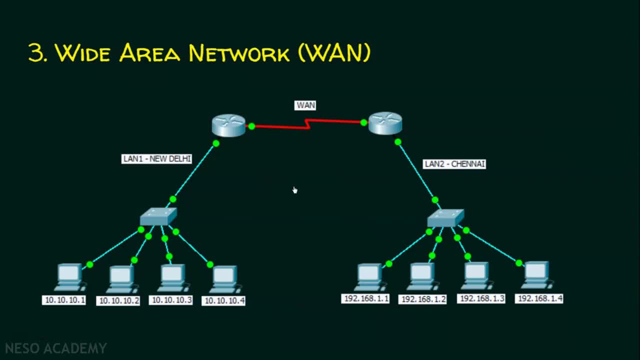 And they are separated by a very large geographical area. This computer can communicate with this computer, And this is possible only with the help of a wide area network. Wide area network means communication at a large distance. If it is a man, this is possible only within a city. 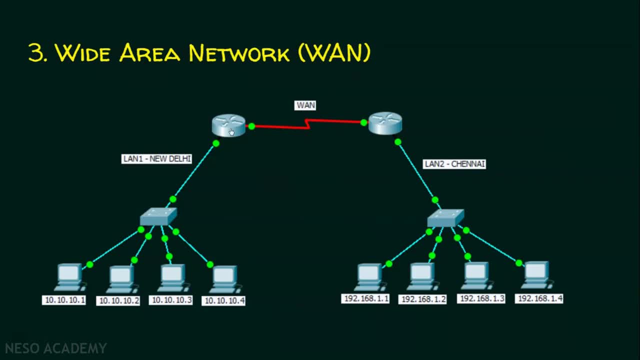 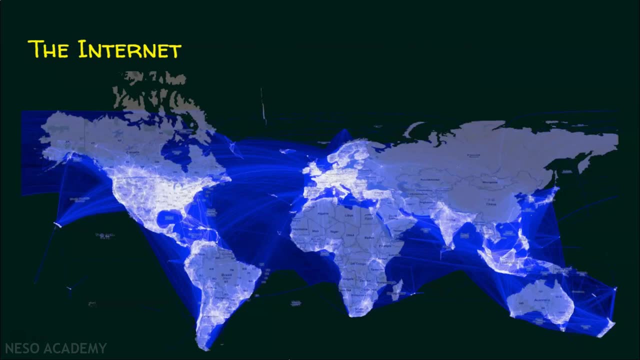 But this is wide area network, hence the communication at a distance is still possible. So far we have seen local area network, metropolitan area network and wide area network. Now we will see the internet. I will say: this is a wide, wide area network. 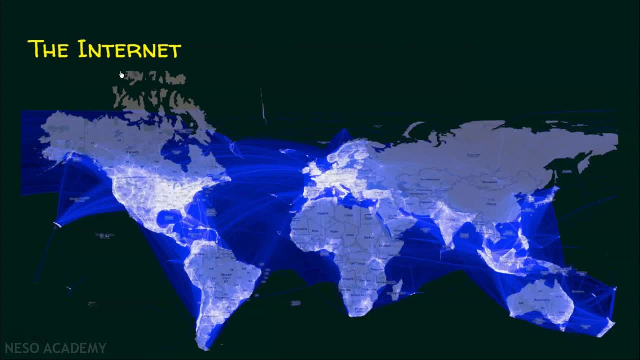 That is a wide WAN. Why? Because there are so many local area networks, so many metropolitan area networks and so many wide area networks across the world are connected to each other. Say, for example, there is a guy in India who wants to send some data to a guy who is in Australia. 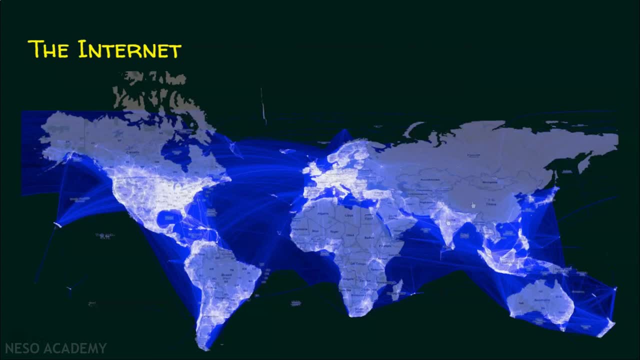 Between India and Australia. there are many routers involved in taking the data from India to Australia. Similarly, every country in the world is somehow connected with other countries through computer networks. We don't know whether two countries have a friendly relationship or not, but definitely they will have a computer network relationship. 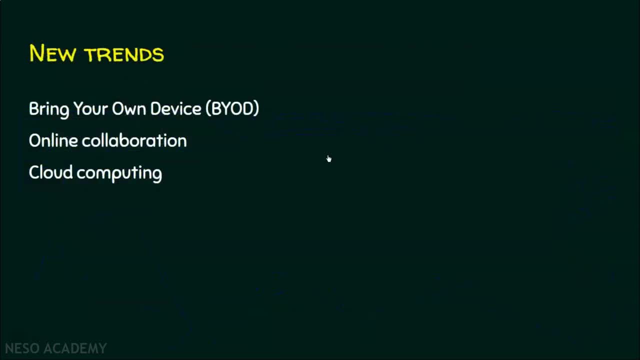 And that's the power of computer network guys. Before we conclude, we will see the new trends in computer networks. Nowadays, many employees are encouraged by their employers to bring their own device and connect to the office network, And we shall call such scenario as a bring your own device scenario. 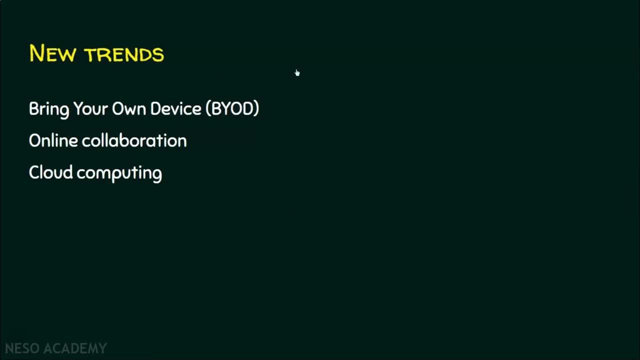 It means employees can bring their own device and connect it to their office network and still work with the office network. Coming to the online collaboration, let's say, at the moment of time, if a meeting is scheduled, everyone has to assemble in the meeting spot. 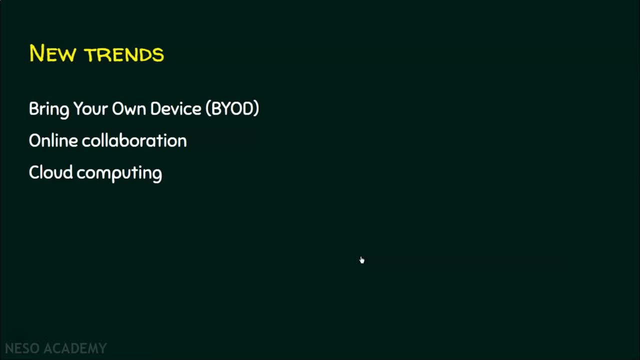 Now the trend has completely been changed. They can participate from wherever they are, and they can still do online collaboration with others with the help of computer network. Say, for example, a meeting involves participants in New Delhi, Chennai, America, Australia, but still no one to be there.